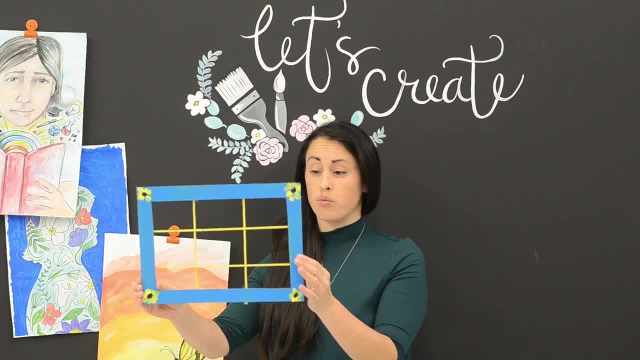 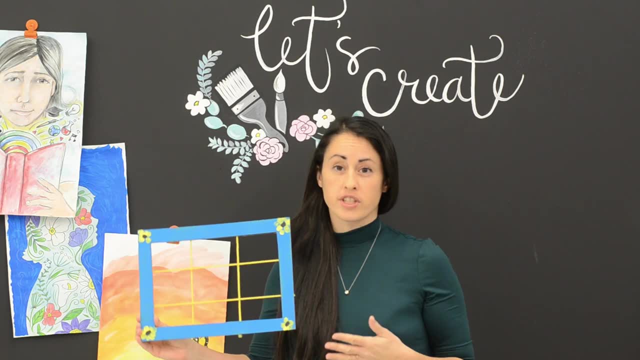 You have four of that, So if you're taking a portrait of someone, you don't want to stick their face right in the middle, but maybe off the top To the side to show a little bit more of your scene in the background. 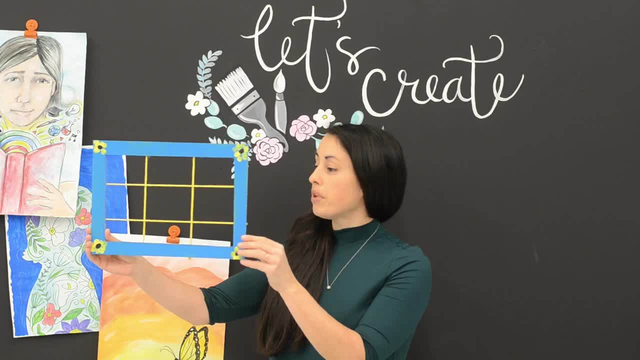 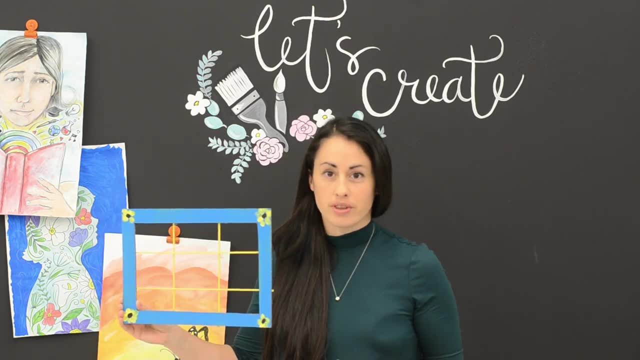 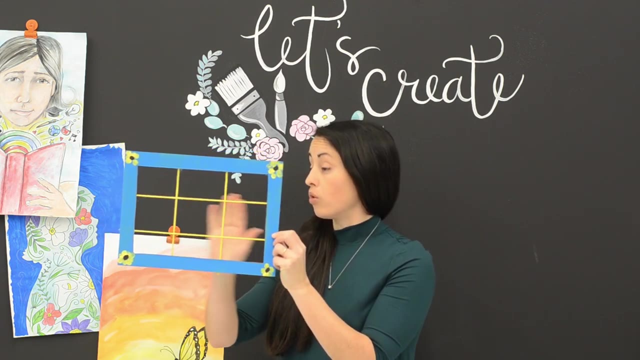 Now, if you're doing a landscape, you want to place your horizon line- And that's a term we use a lot when creating art in my classroom, so everyone should know what that is- But you want to place your horizon line on one of these horizontal lines going across the top or across the bottom. 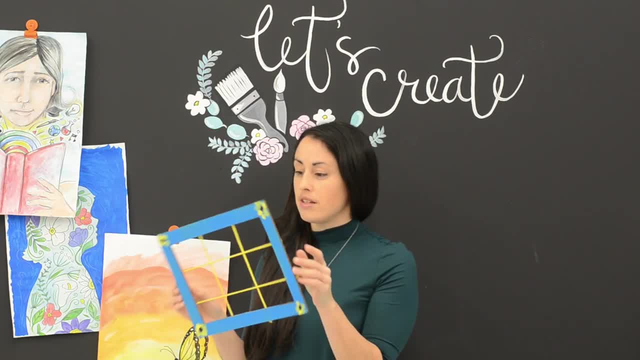 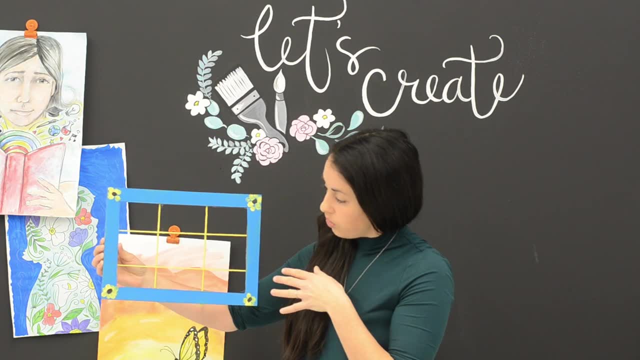 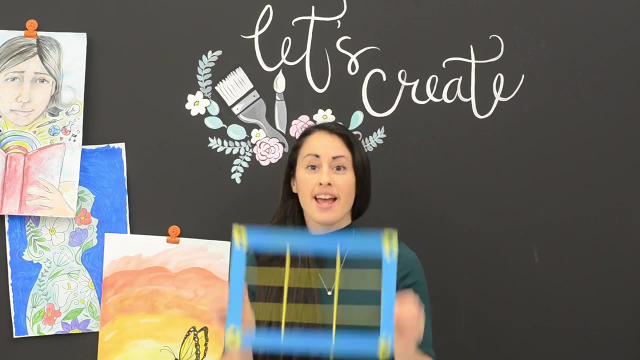 So for our first project together, you're going to be making your own viewfinder With your lines going vertical and horizontal across. Now I'm going to show you all the steps on how to make this fun project, And then you can kind of take it outside and kind of frame up your own shots for a little bit of practice. 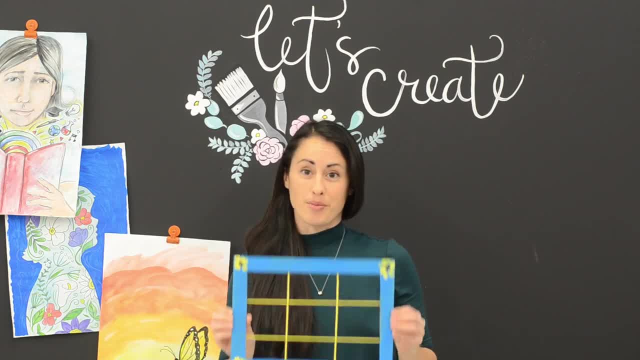 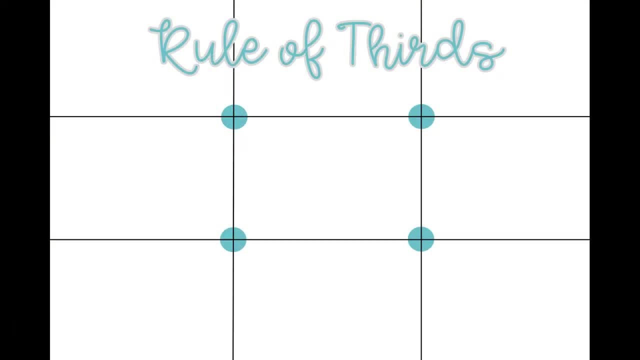 before you kind of dive into using the real camera. So follow along with the steps on making your own rule of thirds grid. Now that you are familiar with the term rule of thirds, let's check out a few examples of the rule of thirds in action. 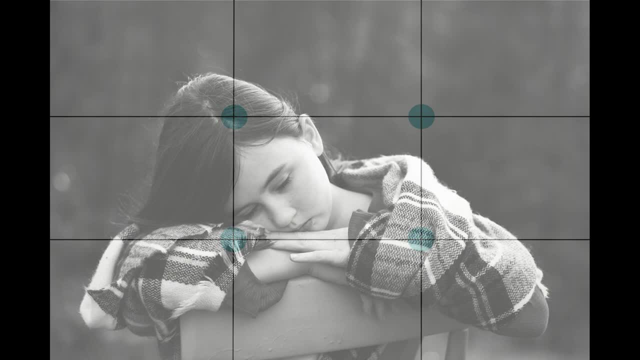 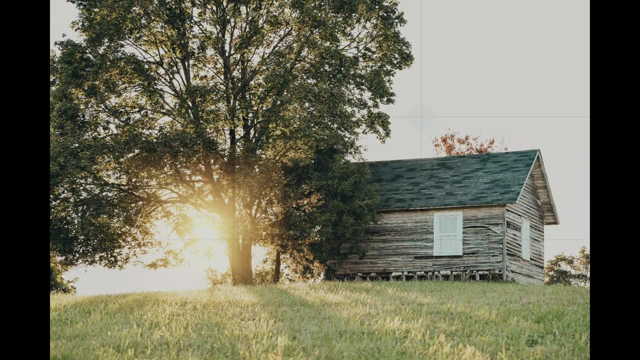 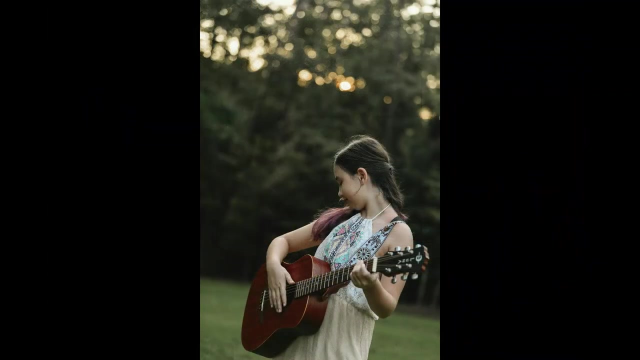 This is my daughter, Ava, and you can see how I lined up her face on the left side of the frame. On this image, I lined up the tree with the two intersecting dots on the left. On this image, I lined up Ava on the three intersecting points. 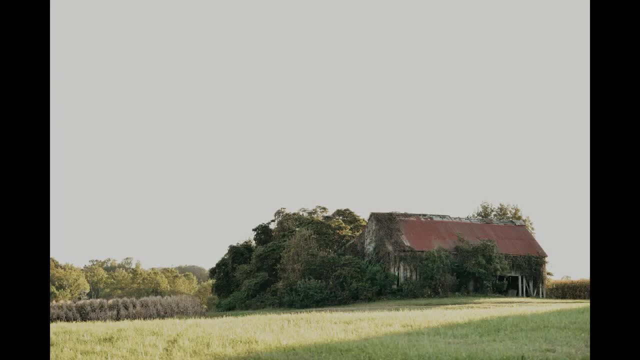 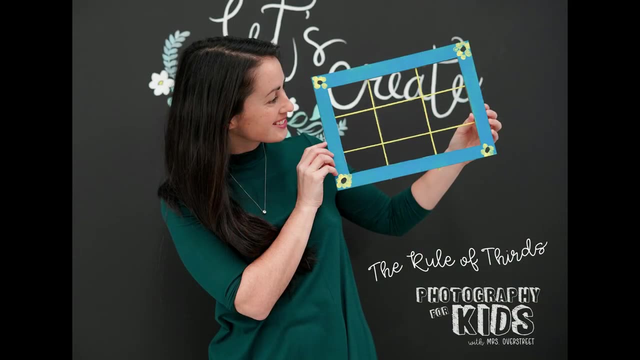 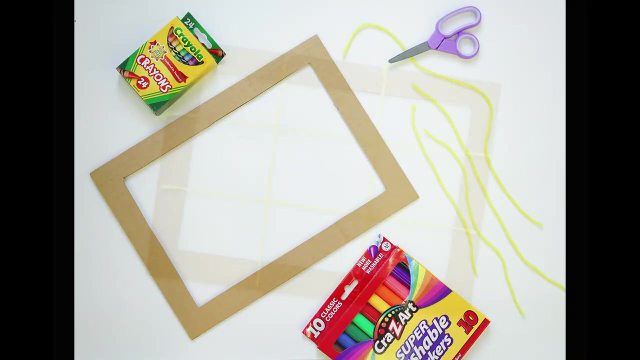 And for my last image, I lined up the barn with the bottom right intersecting point. At this point, I think we're all set to start our grid. All you need is a few simple materials: a piece of cardboard, four pieces of string, tape or glue. 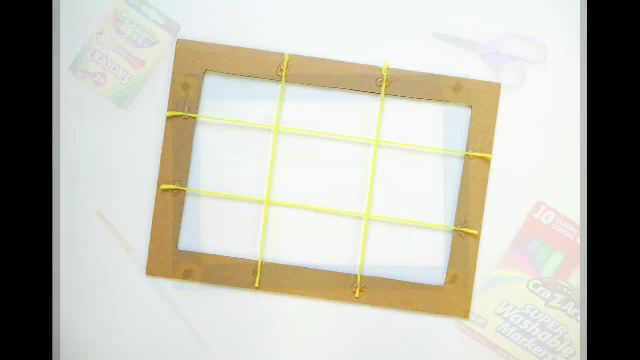 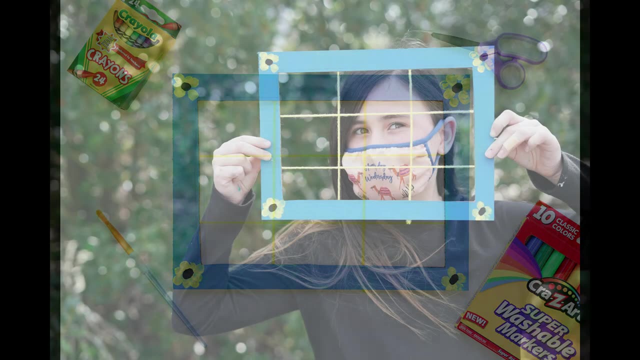 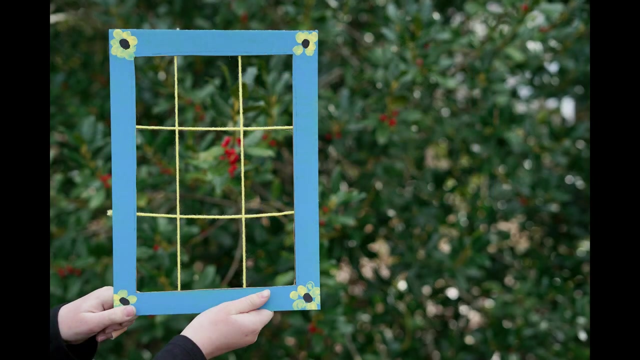 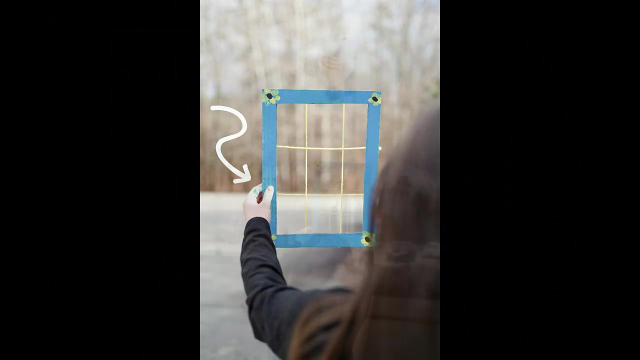 and some coloring supplies to decorate your grid with. Remember, make sure you separate your grid into nine equal boxes with your string. Now let's go out and practice and start framing in the world around us. Before you can take great pictures, you need to know how to create a great composition first. 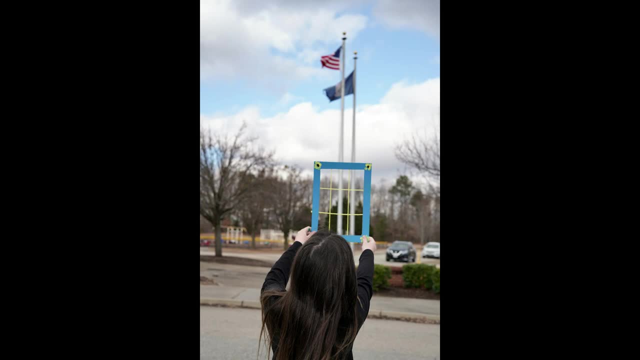 and the rule of thirds can help you do that, As always. thank you for following along at Miss O Art Studio and check back in for more photography lessons.